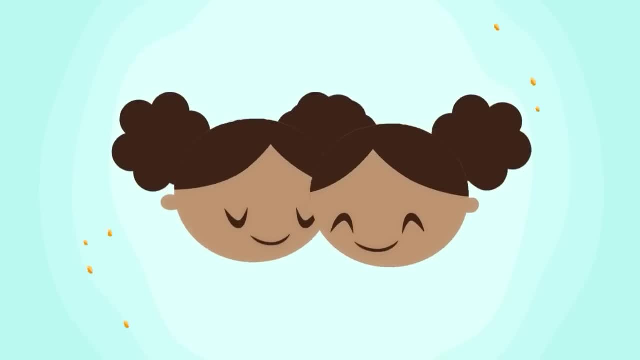 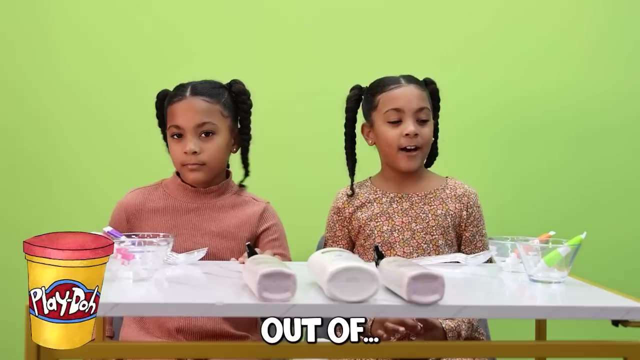 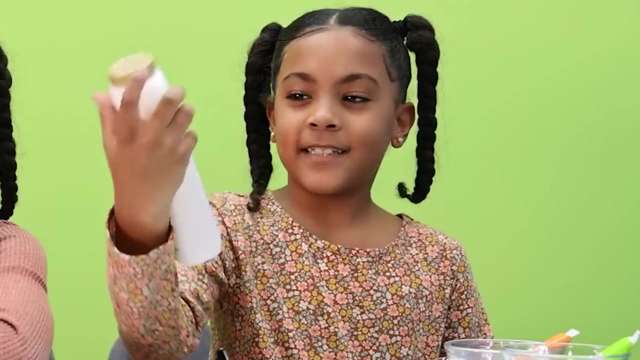 Hi everyone, my name is Ava and my name is Alexis, and we are the McLaughlin's In today's video. well, my sister, she found out a way to make Play-Doh out of. well, these are the materials. We need lotion- any lotion. We need baby powder. This is baby powder. 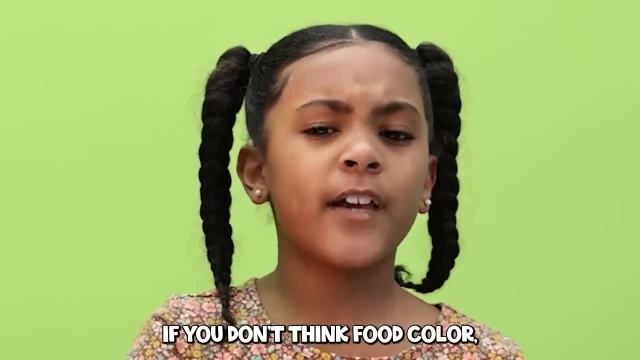 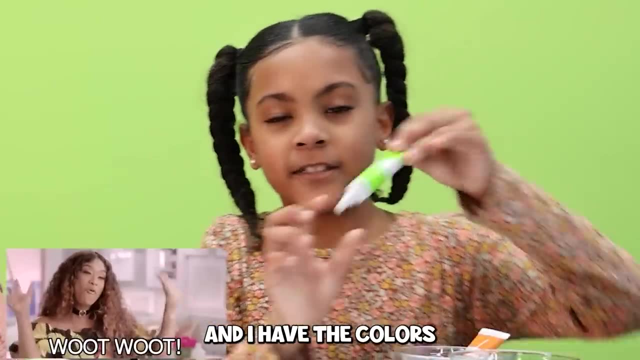 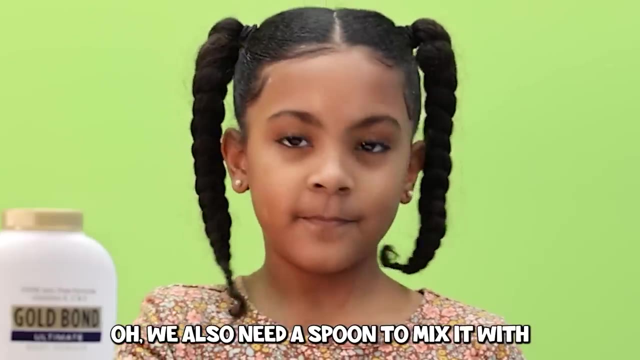 You guys don't have to food color it. If you don't food color it, it would just be white. So I have the colors purple and pink, and I have the colors neon green and orange. So let's get started. Oh, we also need a spoon to mix it with. So the first thing. 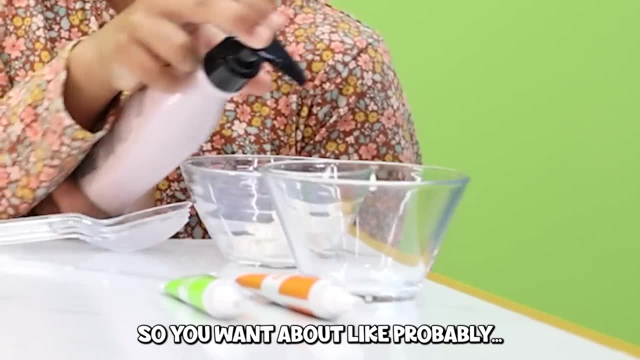 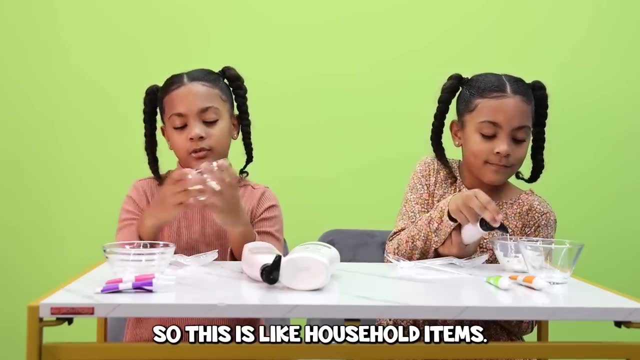 we're going to need is lotion. So you want about like probably 10 squirts. Do this one A little bit more So you want the whole. That's enough, That's enough. So this is like household items. So most of you guys probably are already going to. 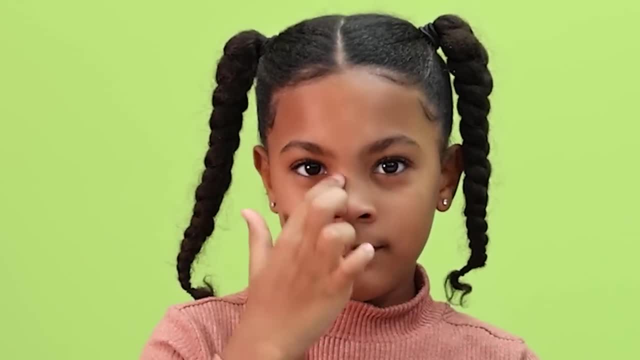 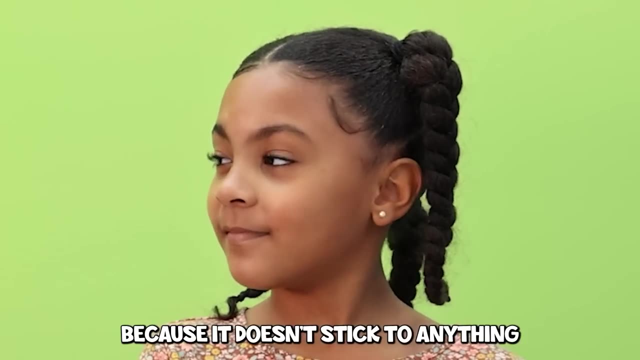 have baby powder and lotion And cups at home, Spoons, of course. This also like it's good because we've made it before but not on video. It's good because it doesn't stick to nothing. It dries out like very quickly, So you might want to. 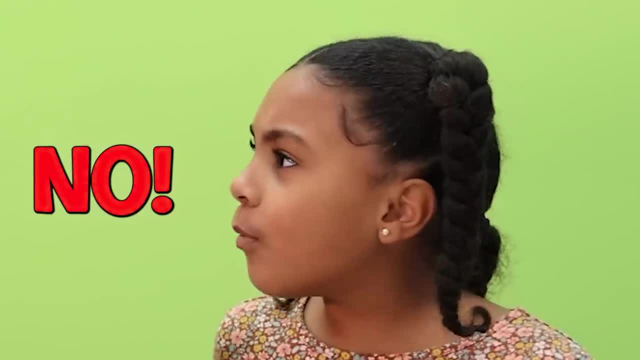 put it in a moist Ziploc bag. No, Dump the water out. No, That is not how you do it. And then put the putty in. So do not put the water in the bag. Yes, do it. I did not do that. 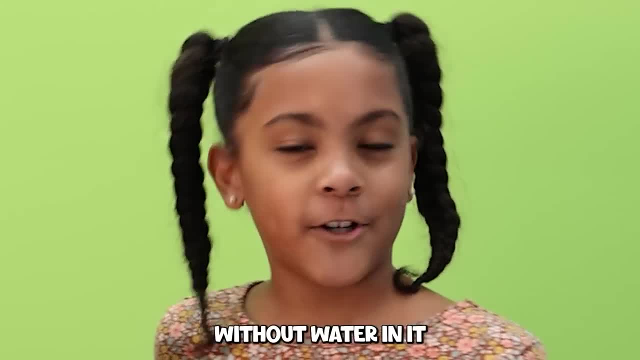 You should do it. You should put it in a container or a Ziploc bag without water in it. Put it in a moist container or Ziploc bag. No, No, Alexis. Okay, So the second thing we need to do is put baby powder in it. 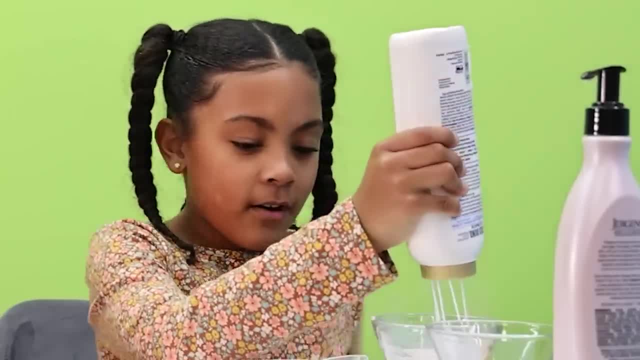 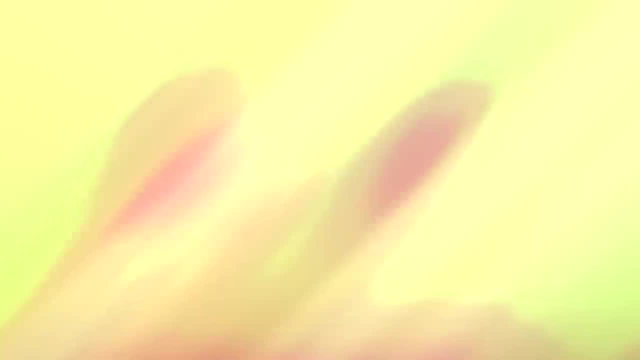 Wow, A lot of baby powder. Okay, A lot of baby powder. Now she gets baby powder. Now, what we're going to do is we're going to get lotion, a little bit more lotion, and we're going to squat. 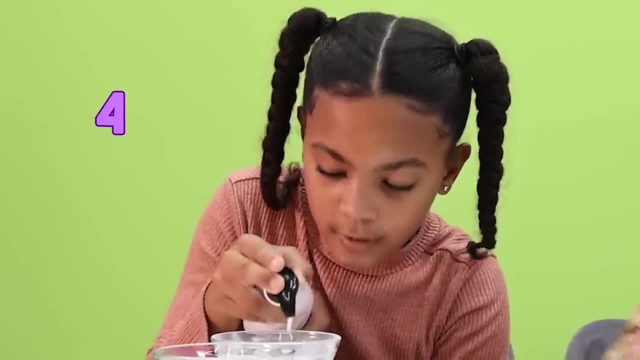 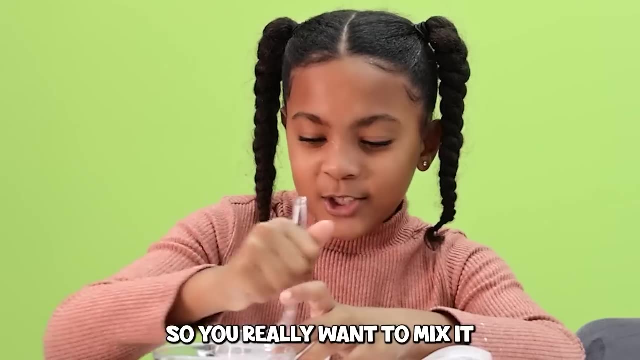 One, two, three, four, I mean six, seven. So now we want to put the food coloring in it. No, But we need to mix it a little bit. So you really want to mix it. You really want to mix it like really good, and if you put too much powder, put more lotion. 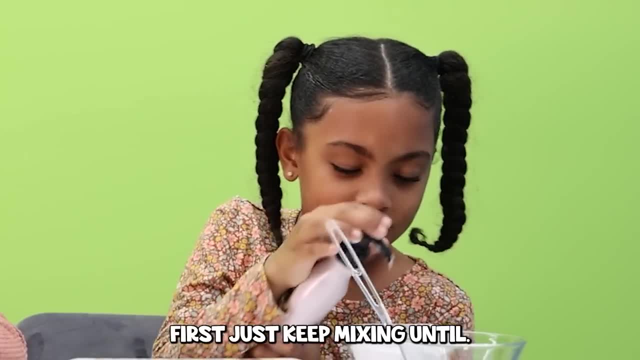 and it's going to mix it. Yeah, So I'm going to put more lotion, But if it doesn't work at first, just keep mixing it and then at some point you need to form it with your hands, but you need to mix it. 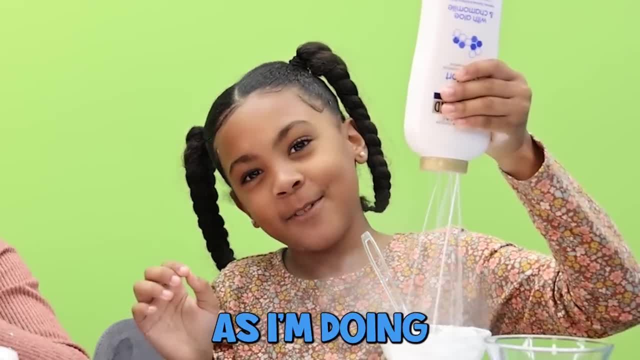 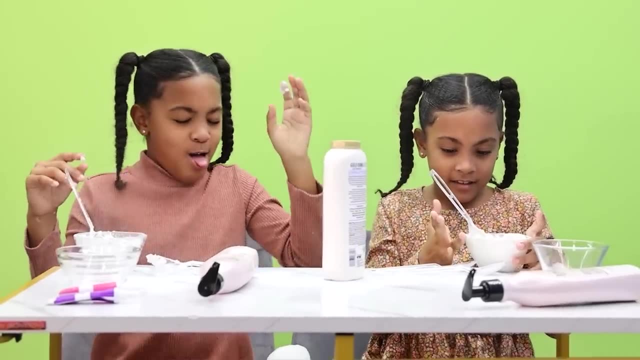 We have to just get it more thick. You have to add lots of baby powder, as I'm doing, and Okay, Okay, You can use all of it. There's barely any baby powder in here. Okay, Ow, This is not toxic. 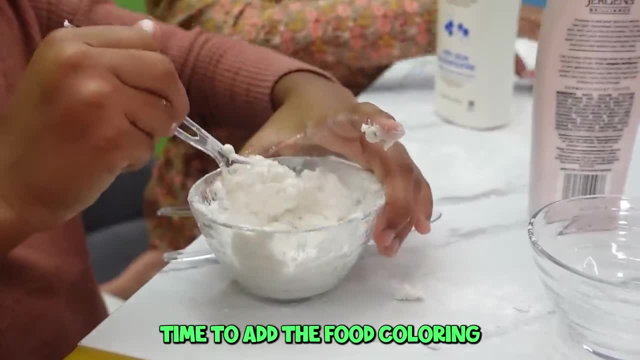 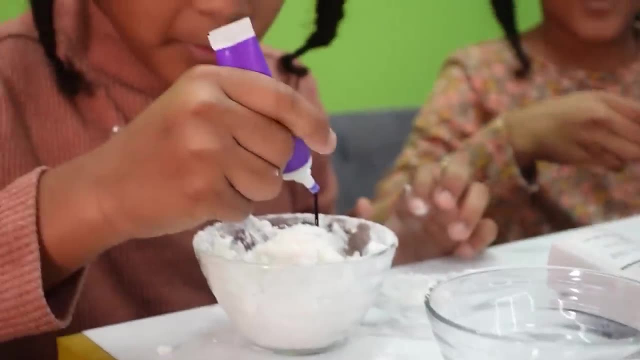 I got scared. Okay, I think it's now time to add the food coloring. Yes, Okay, Okay, I'm going to use the orange Purple. I'm using the purple. I'm using the orange. Okay. So what I'm going to do is just going to like. 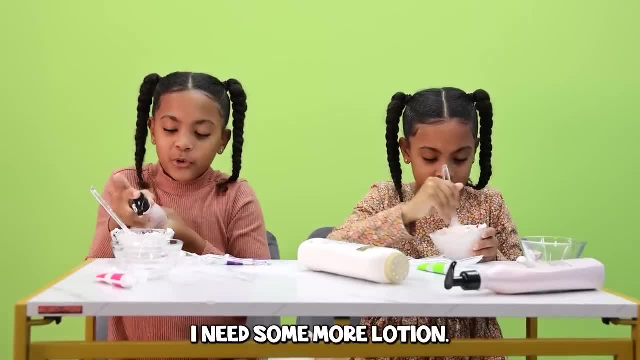 Do the squeeze. So that's all I want for now. I need some more lotion, Whoa, Okay, So we might need to use the whole bottle. so I'm sorry, I'm adding a lot. This is going to turn into red. 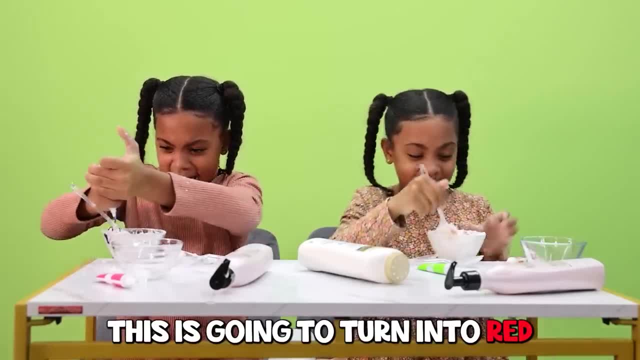 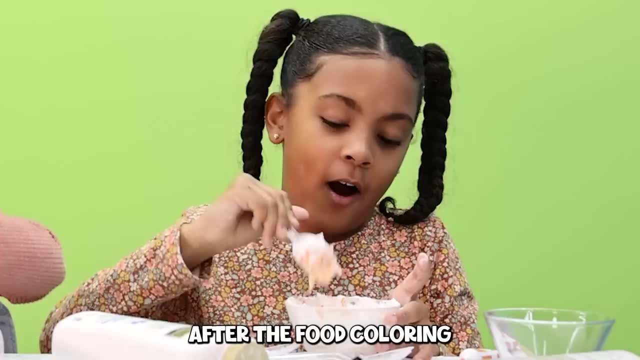 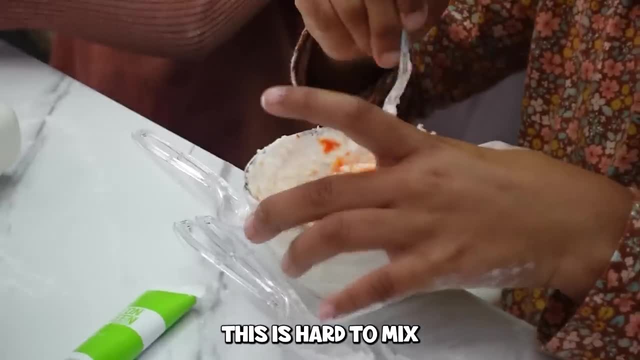 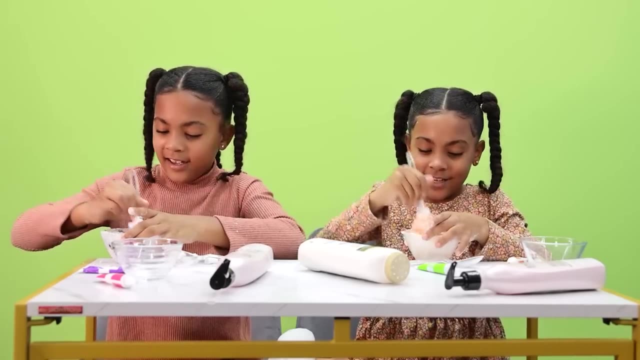 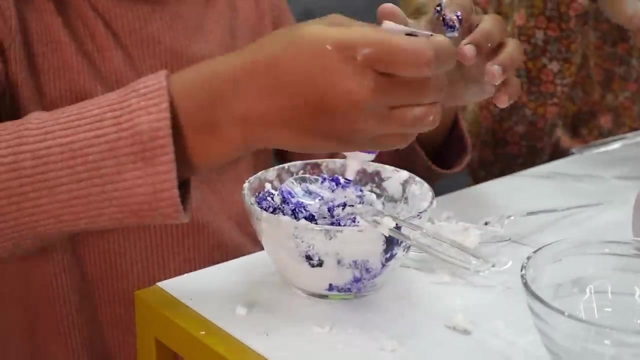 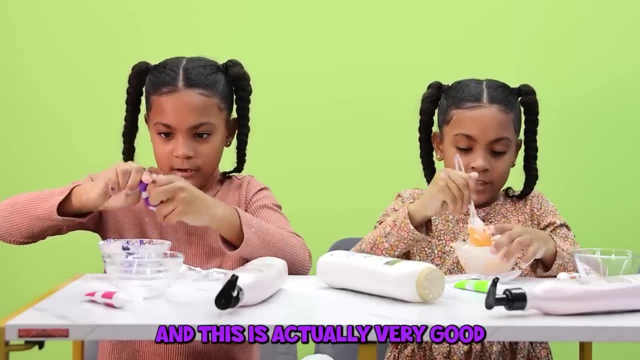 Okay, Okay, Mine's turning out very good. I think it's turning orange Okay. So what I'm going to do is- And this is actually very good, Alexia, I actually made it orange Cool, I think yours is better than mine. 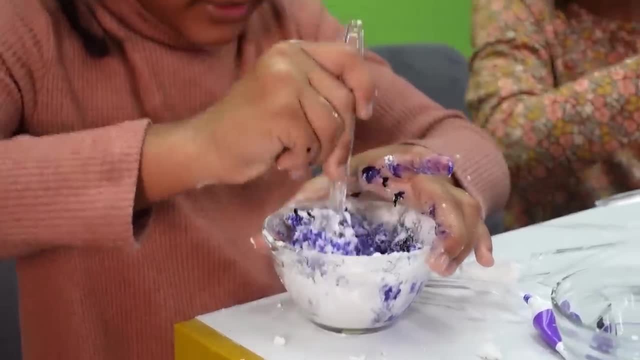 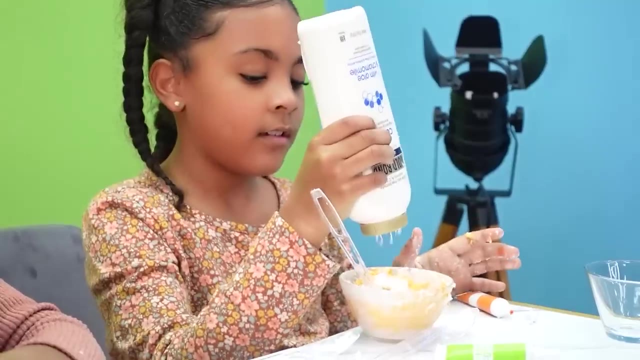 All right, Gosh, yours is pretty orange. Alexia, We need to mix it with our hands, Our hands, Right now. Yes, That's what Baby Project lost Me? Yeah, Why me? Okay, Ava, stop, it's mine. 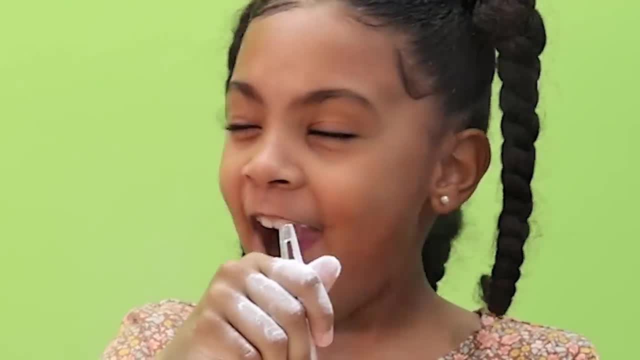 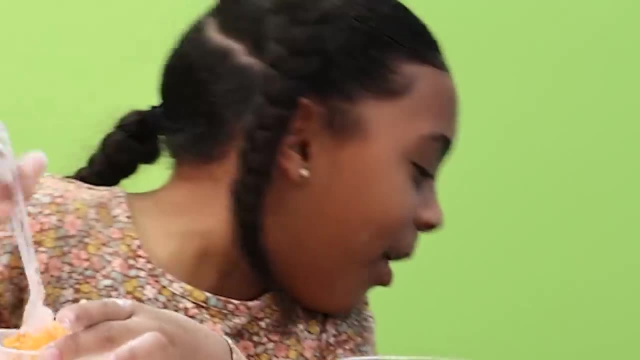 Okay, so now Did you get from messing up mine. Well, I didn't put a lot, All right, close that thing. It's kind of a tonic blue. Oh, my gosh Blue. Yeah, you see some blue in there. 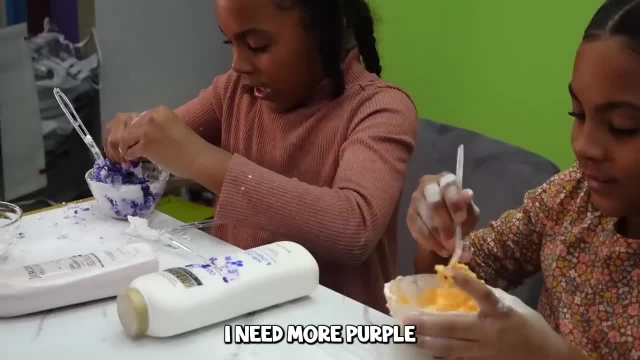 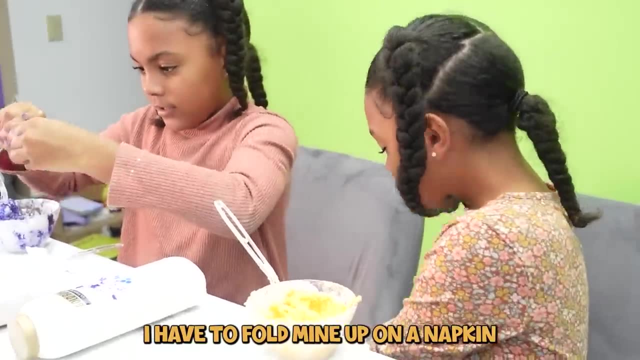 Mixing it up. Okay, it's working. it's working. I need more purple. I want it to be like so purple. Okay, I think that way I have to form it up on a napkin. I have a napkin. 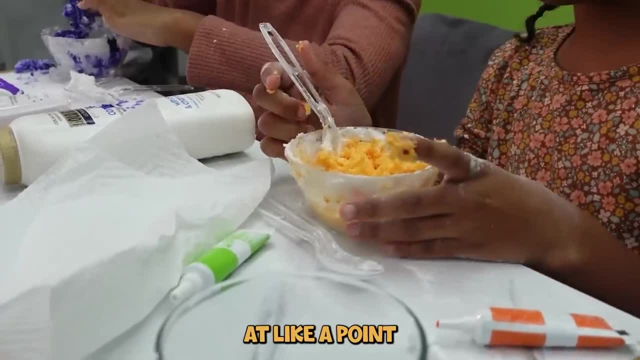 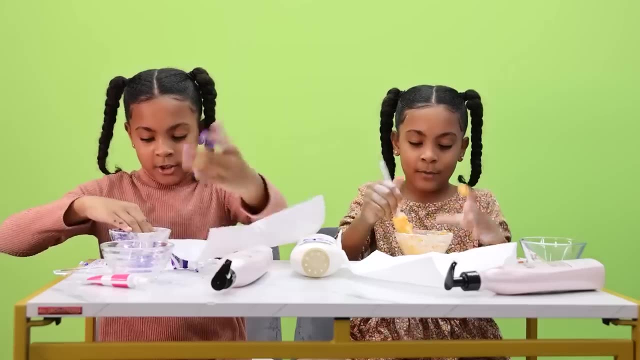 So the napkin is for the forming up. So after like a point it's close on the Play-Doh, you want to start like taking it out of the bowl or cup or whatever and start mixing it with your hands. So what I'm gonna do is just gonna. 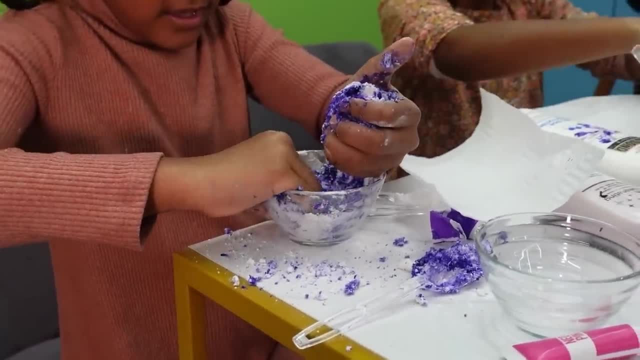 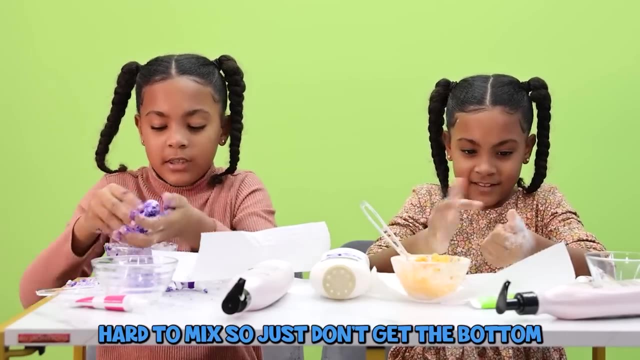 I'm gonna get a giant scoop. Yeah, let me try. Okay, okay, giant scoop. Guys, the bottom is the one that's really still like hard to pick, so just don't get in the bottom. By the way, guys, you can't roll this like this. 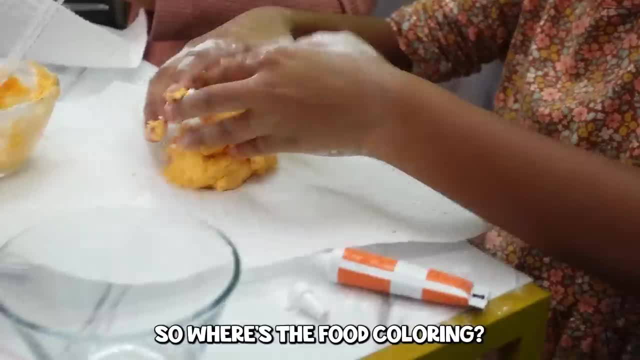 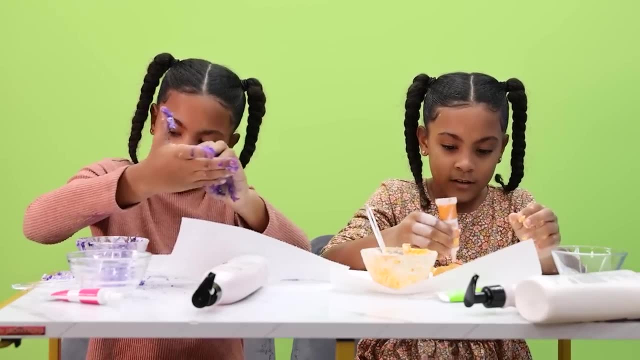 because then it'll mess it up. Okay, I'm gonna take a bunch, So where's the food coming? So I want to get some more food coming. Now I'm gonna add a little bit more food. I really wish I wore gloves, but you know. 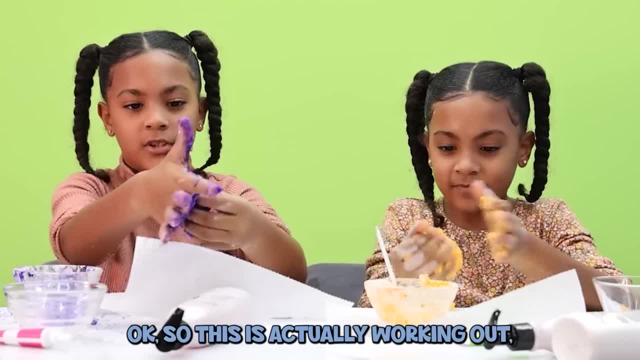 Oh my gosh, I'm gonna mix the food. Could somebody roll my sleeves up? Okay, so this is actually working out, So you might want to let it dry for a little bit. But, guys, if this is not good for you, 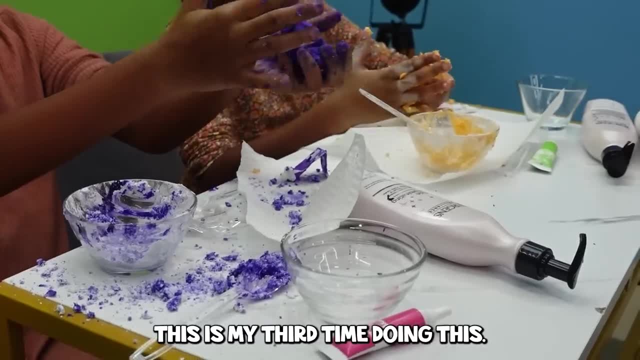 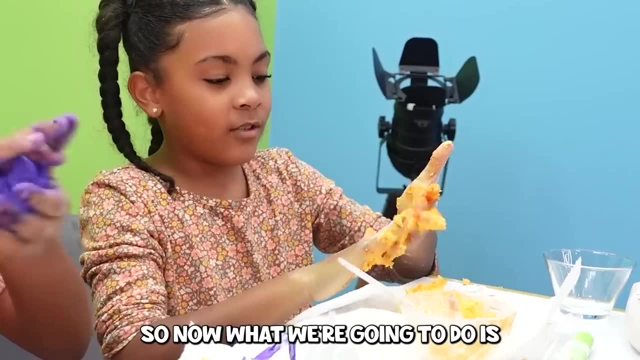 then you're doing it wrong. okay, Because I did it three times. This is my third time doing this. You know why? Because I did it last night two times. By the way, you have to add lots of powder. This is not done yet. 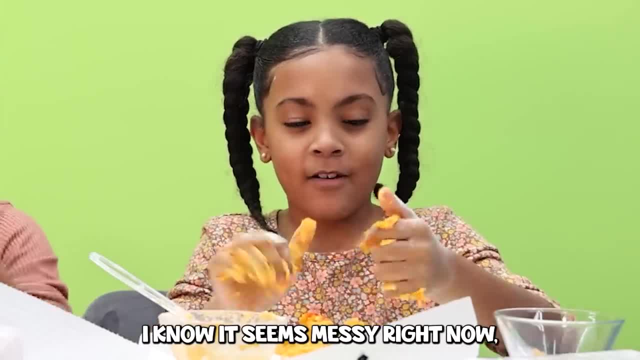 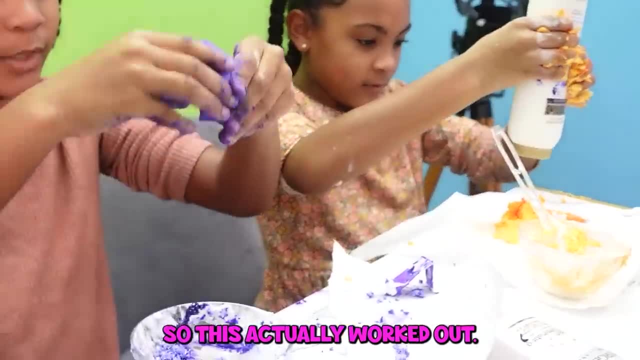 So now what we're gonna do is- I know it seems messy right now. I'll wash the baby powder off. Oh my gosh, oh my gosh. So this is actually worked out. Look at this, this: How do you open this? 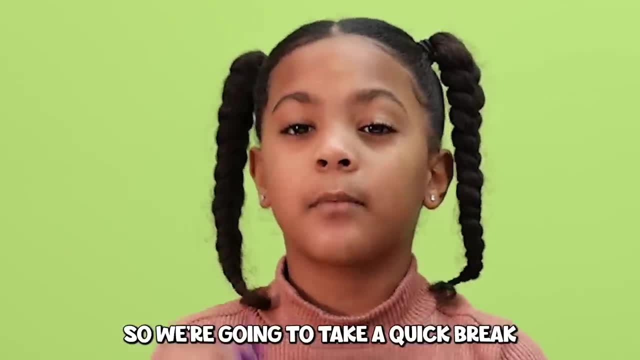 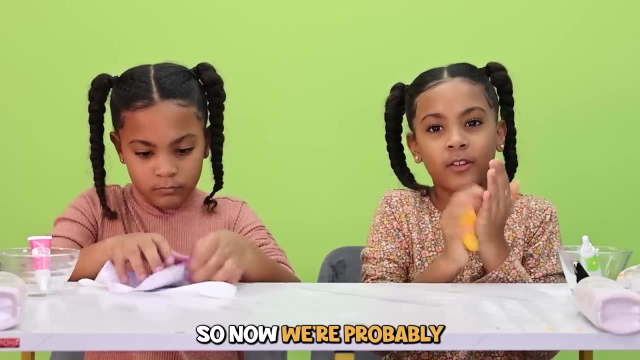 Okay, now we're gonna put a little bit more. So we're going to take a quick break so we can clean up, and then we'll do the next one Two hours later, Two hours later. So now we're probably gonna make. 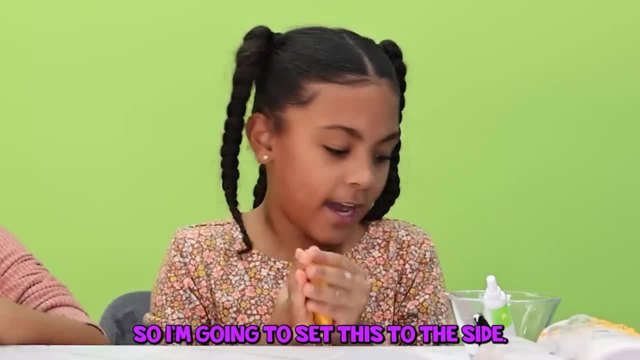 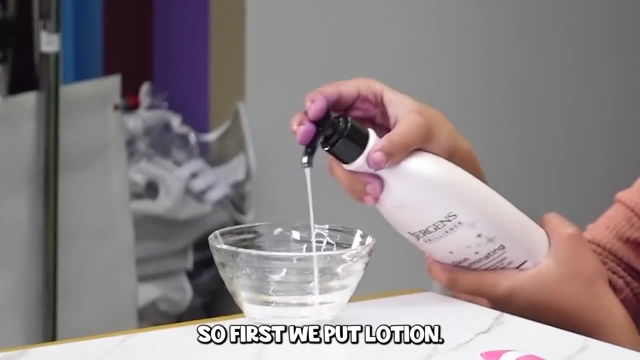 a different color right now. So I'm gonna set this to the side. I'm gonna put this on a napkin. Okay, guys. so we are ready to make the second one. So first we put lotion, A lot of lotion, guys. 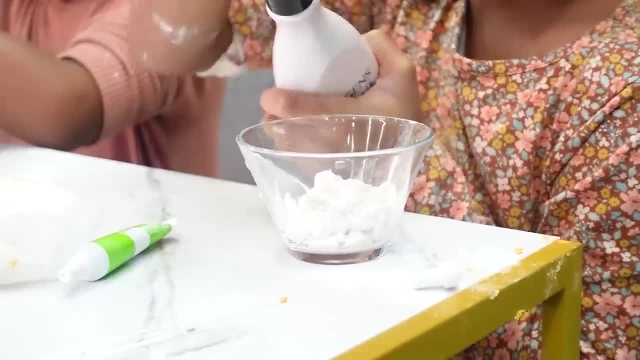 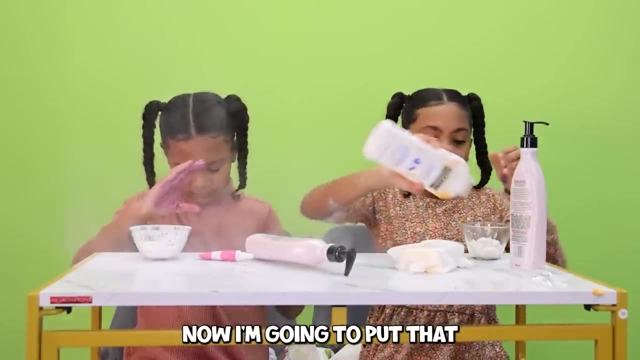 Like maybe fill in the whole bottom, I'm still putting it: Okay, now I'm gonna put, oh my gosh, that's a lot. There we go. Now I'm gonna put that: let's see, There's barely any more like this: 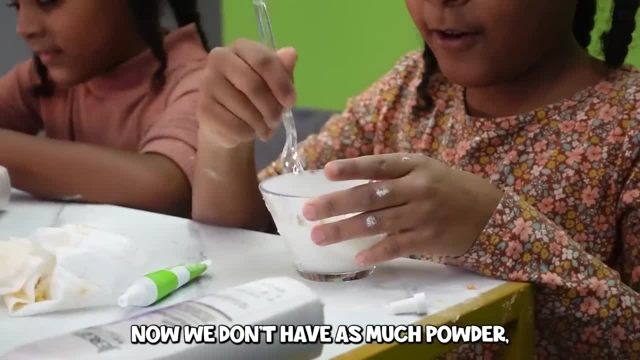 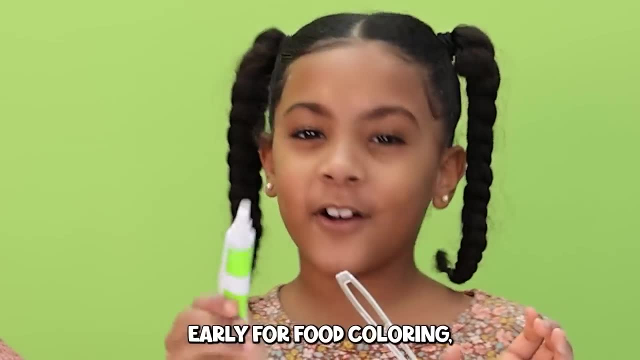 Now I'm gonna mix it Now. we don't have as much powder, so it might end up a little bit more slimy. That's okay. We don't really have enough sense. This is a little bit oily for food coloring, but I'm gonna go ahead and put it in. 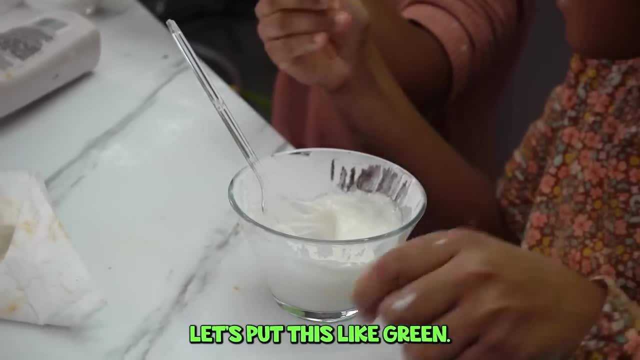 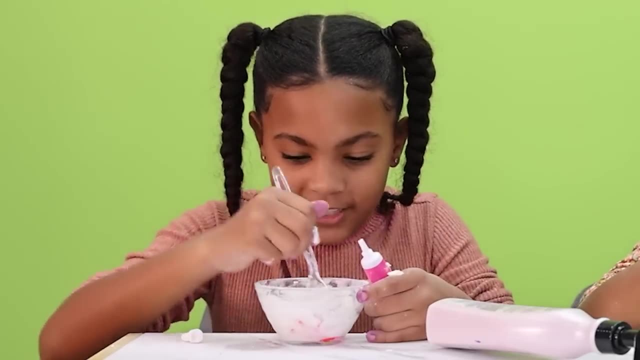 because I don't think there's anything else I can add to it. So let's put: I'm gonna put green. Okay, ready, Oh my gosh. This pink is so pretty. Wait, is it? Oh my gosh. 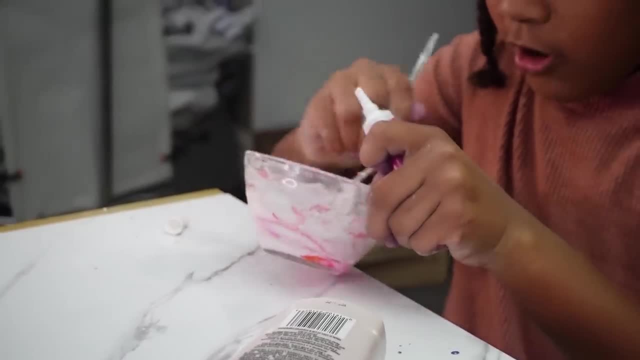 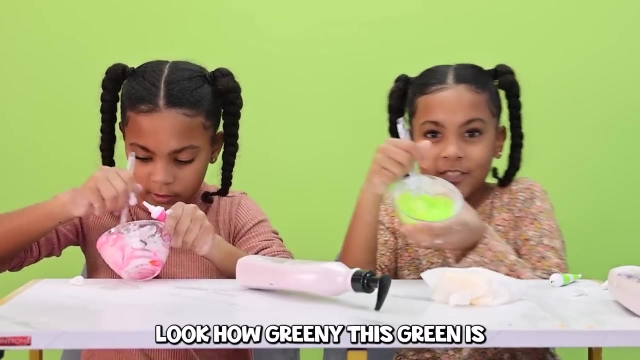 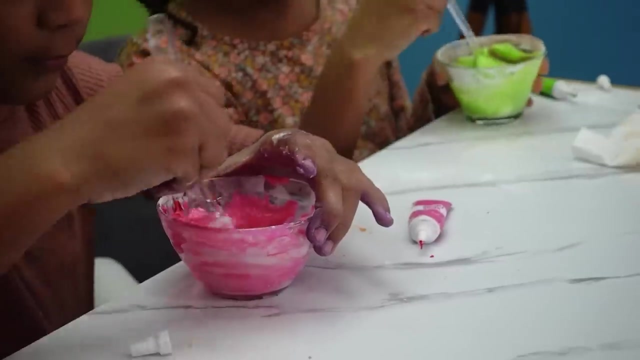 Yay, this is so pretty, I'm gonna put it in now. Wahoo, Now this green looks good. Oh my gosh, look how creamy this green is. It looks like icing. look, So yeah, and just mix it up. 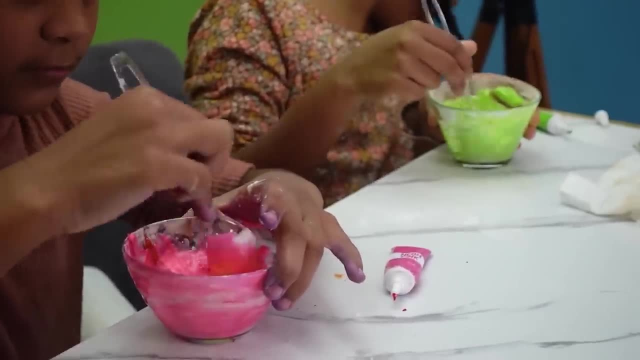 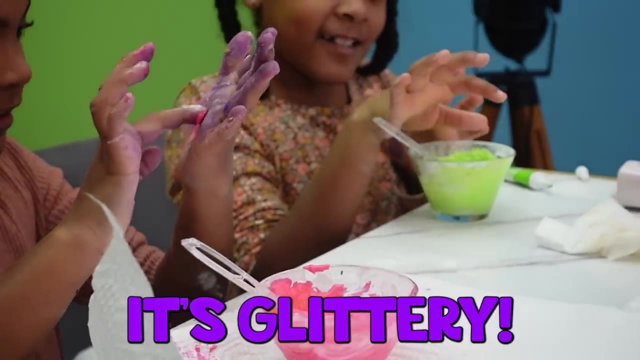 Mix it up. So this is what it smells like. It smells like lotion. because it's lotion, It smells really good. Take a little bit of the rub in my skin, because it's lotion. It's glittery. I'm gonna see, since it's lotion, and it'll rub. 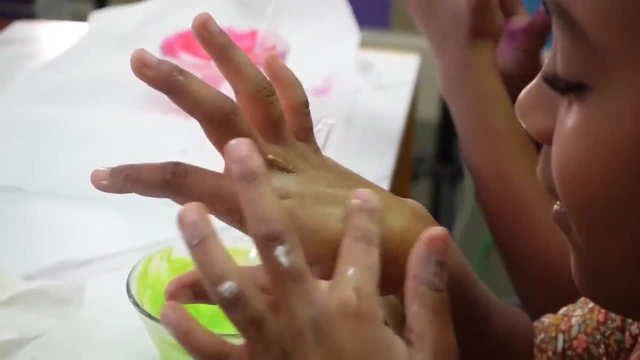 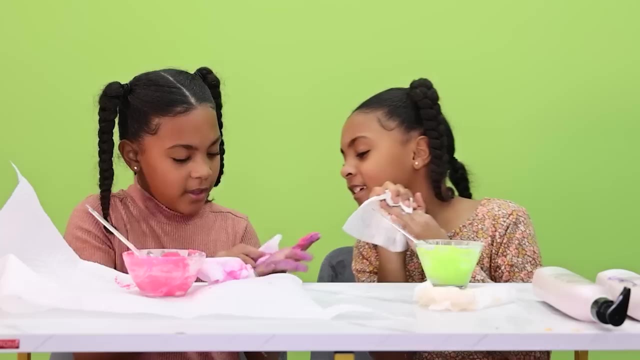 It's like, it's like it gets to pop a lot. Oh my gosh, This is definitely not what I need. All I need to do is like rub it on there and then get a wipe And then wipe it off. Alexis. 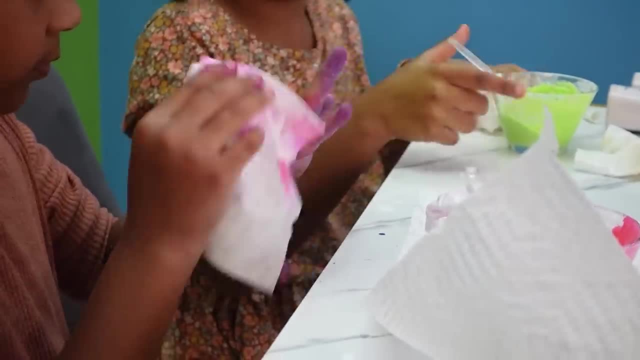 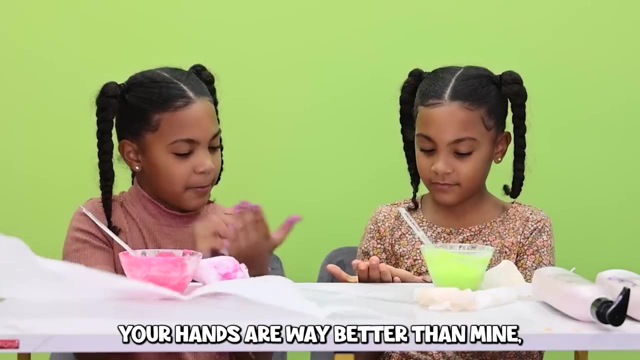 And then bam, What is wrong with you? Didn't knock over at all, Alexis. why would you put the pink all over your hands? I don't know, Because you're crazy. Let me see your hands. Your hands are way better than mine. 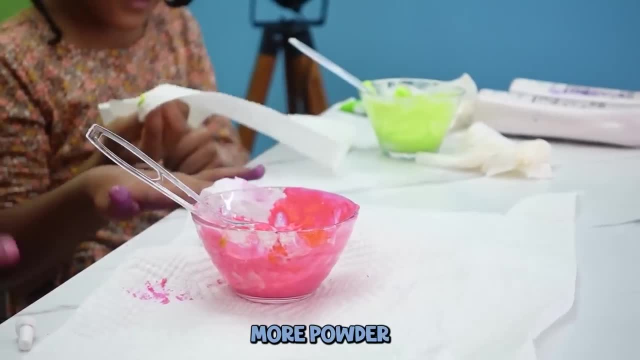 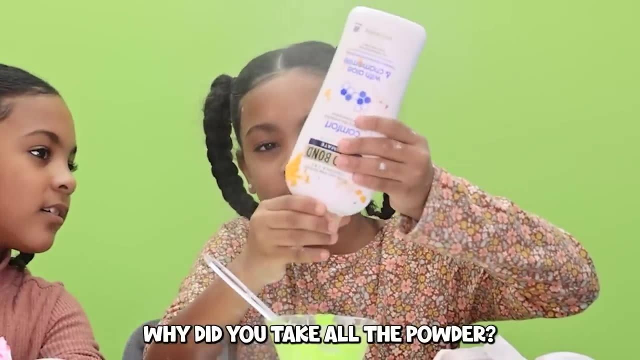 because you picked orange. I think we actually need more powder. There's no more powder, There is, There's more. Okay, So now we're gonna add a little bit more powder. Alexis, why did you take all the powder? Because mine's more liquidy. 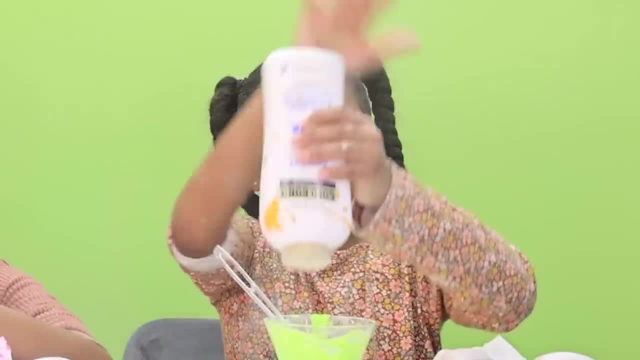 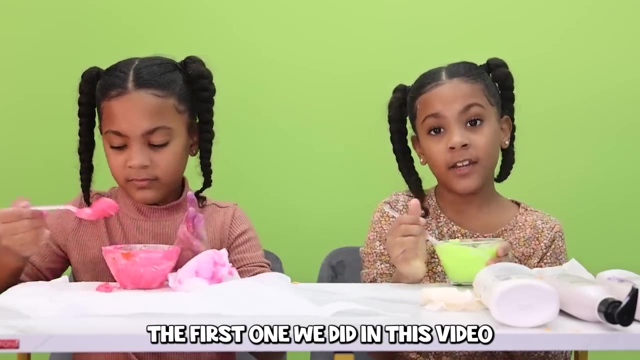 It even looks like the Nickelodeon slime. I'm gonna add as much powder as I can. This is not working out. So, guys, this slime actually isn't working out. The first slime we did in this video. those worked out way better. 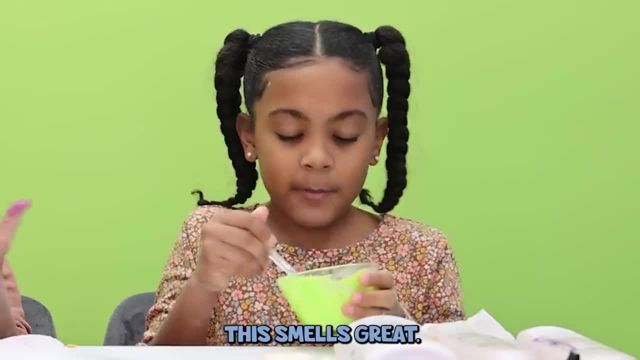 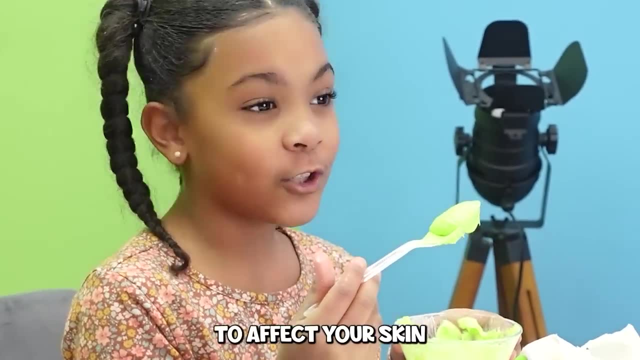 but we didn't have the powder, So this doesn't smell good. This smells great. Oh my gosh, You know where you can use this If you want it to turn green, if you want it to affect your skin. it might be the hope. 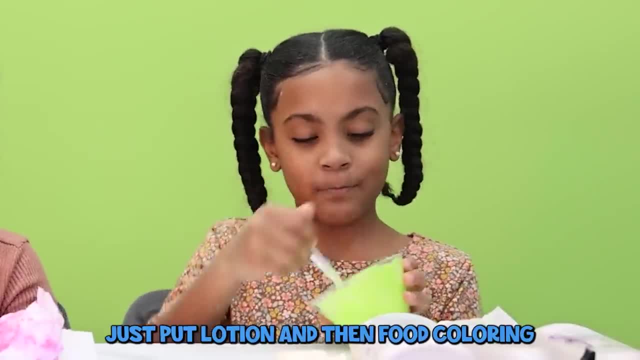 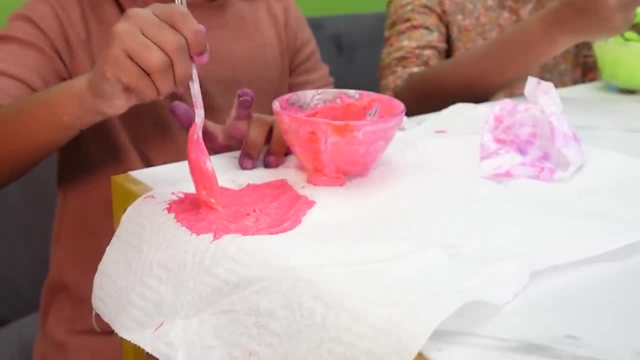 but you don't want to put paint on your skin because you think it'll look bad. Just put lotion and then food coloring. It can go in your body. It can probably go on your body. So all you have to do, and then you could just make the eyes like that. 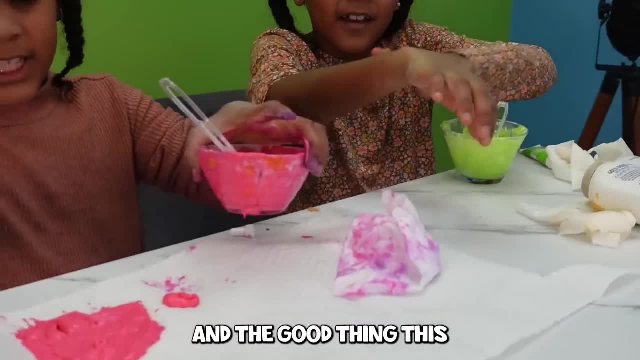 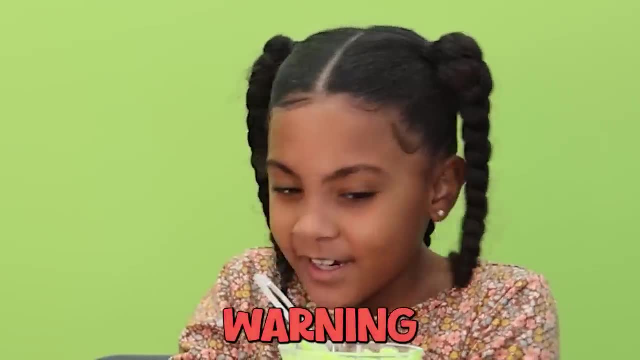 and then rub it Ta-da. And the good thing, this does not go through paper towel, Does it No? No, But, guys, Warning, You may want to ask your parents to do this before you do it, because it might make a little bit of a mess. 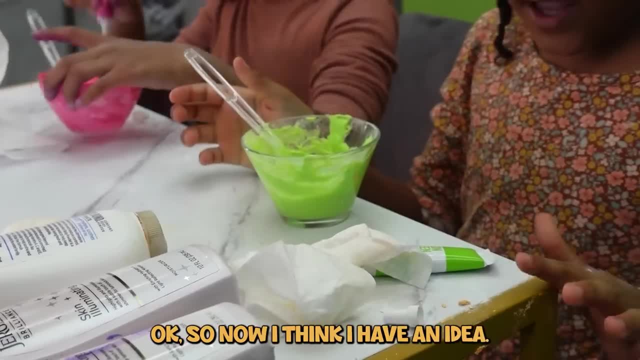 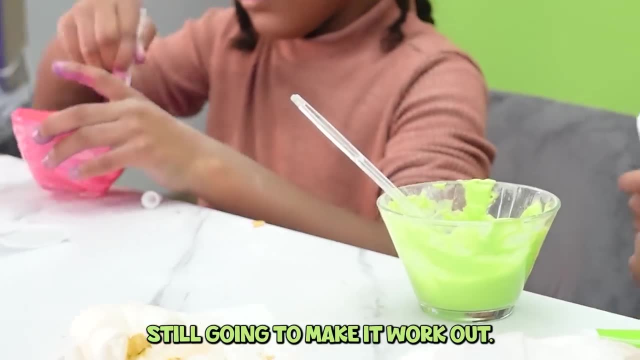 No, Nobody likes when you get in trouble. Okay, so now I have an idea. Okay so this didn't work out, But the second one, We're still gonna make it work out. Get paper towel, Alexis. I have an idea. 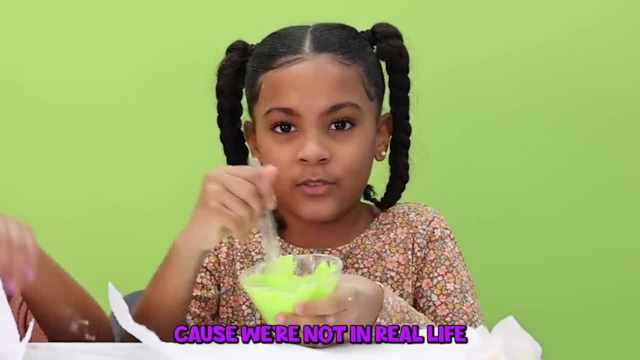 And you see this is very watery. You might not see it because you're not in the light. So do you like put the paper towel in? So I'm going to double up the paper towel like this. So you put the paper towel in the 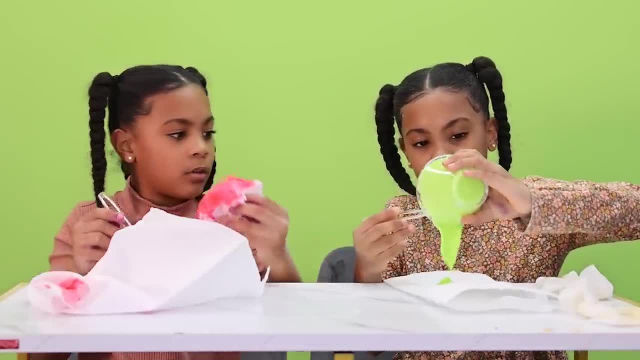 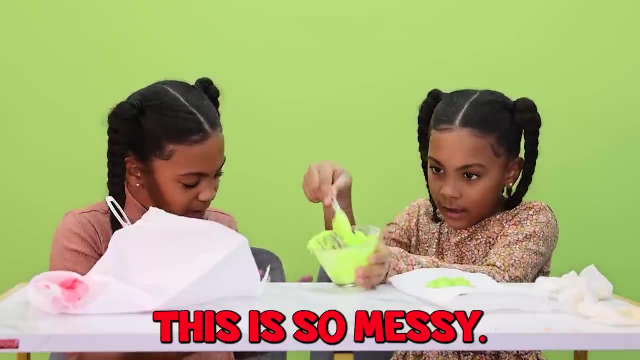 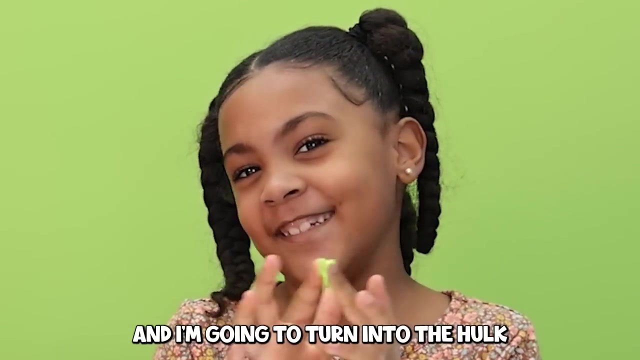 No, I'm gonna pour it. What are you doing? I already did it. I'm gonna pour it. I need a wipe. This is so messy. No, I'm going to take a scoop of it with my hand And I'm gonna turn into the Hulk. 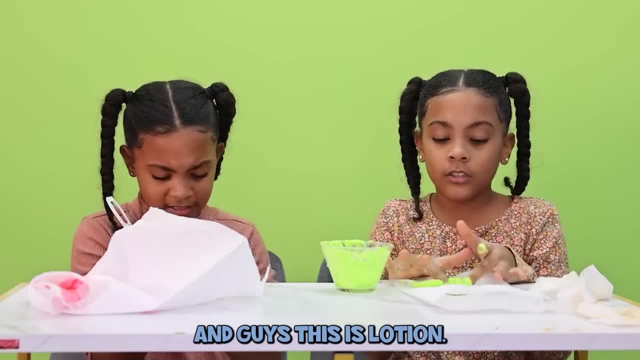 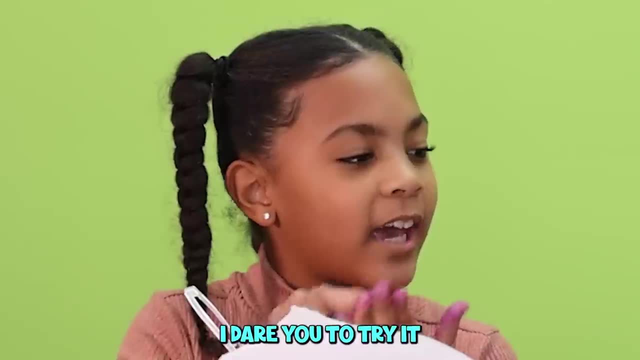 And this is how I'm gonna do it. And, guys, this is lotion. If I can eat food coloring, then I can probably put it on my face, because the inside is part of my body and the outside is part of my body. Okay, there, you try it. 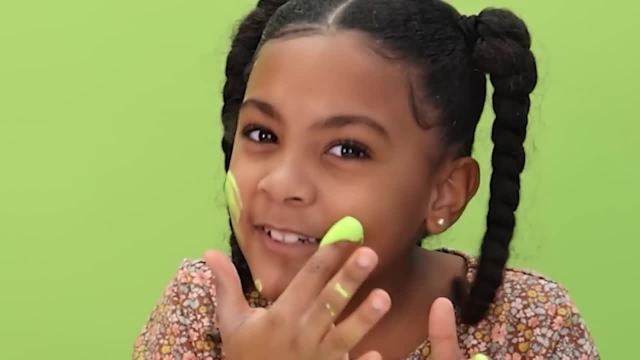 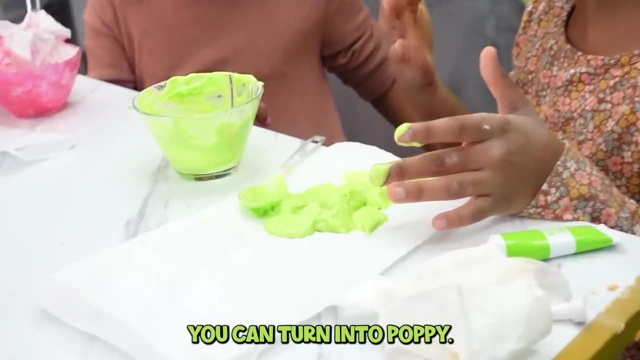 All over your face. All over it. Keep going. I wanna turn into the Hulk. Can I help you rub it in? No, You do it yourself, Alexa, you can turn into Poppy, Poppy, I don't wanna turn into Poppy. 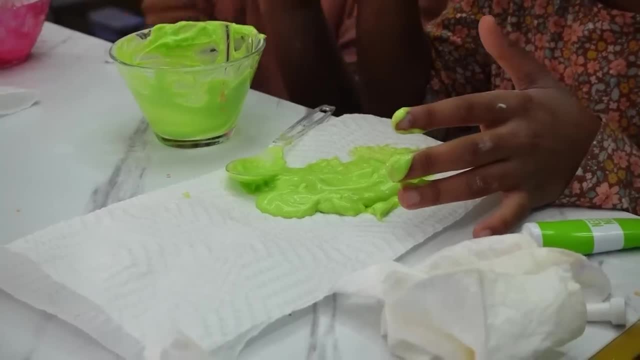 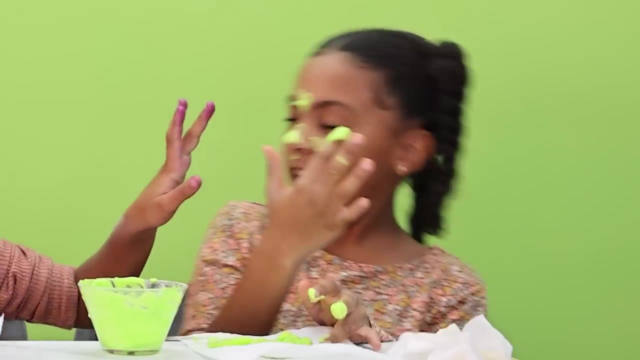 Ava's gonna see your face? No, it's not. Look at my hands. I look like a huh, I look like a Hulk. now, Guys, I won't be doing this because it's not working out, So it's another thing to do. 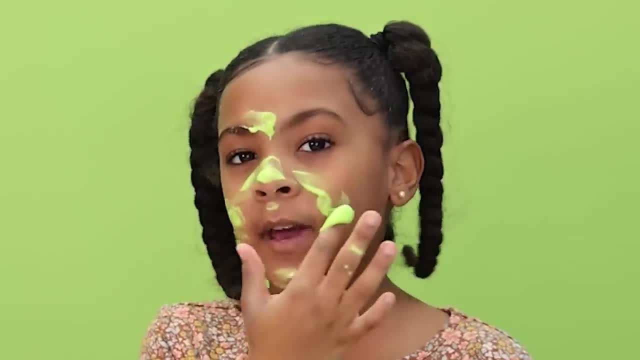 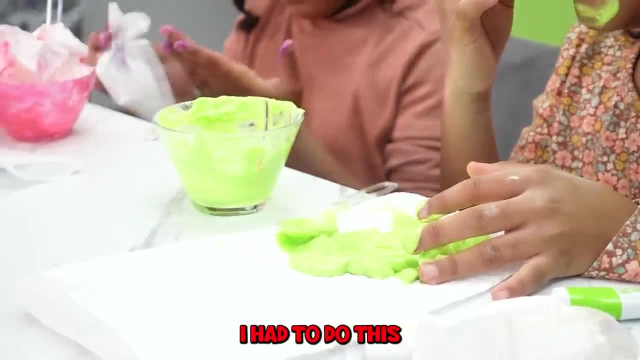 Hey, Don't not touch my face. By the way, don't trust for somebody else to do it on your face, because they will probably make you look crazy, Just like Alexis. One time at this birthday party I had to do this and it smelled so bad. 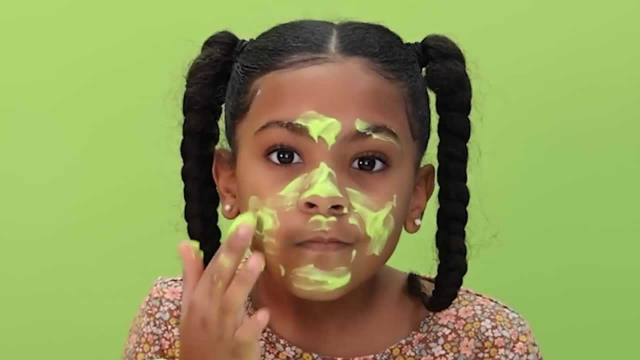 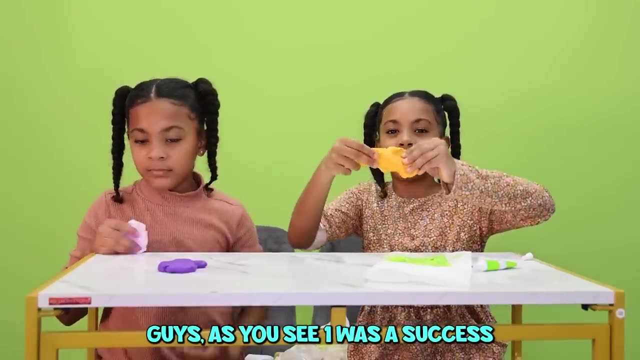 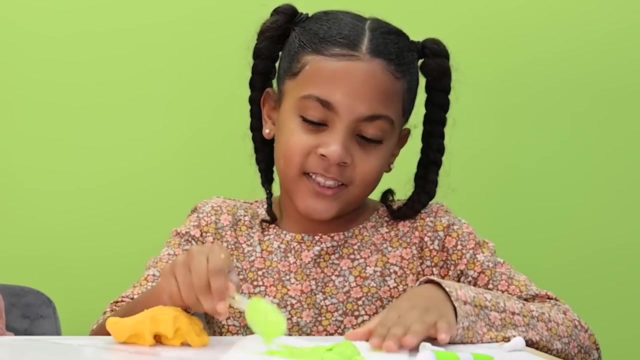 But this one is lotion, so it smells good. Okay, I think it's kind of coming off, Guys. as you see, one was a success. The first one was a success because we had enough powder, But the last one you should see. 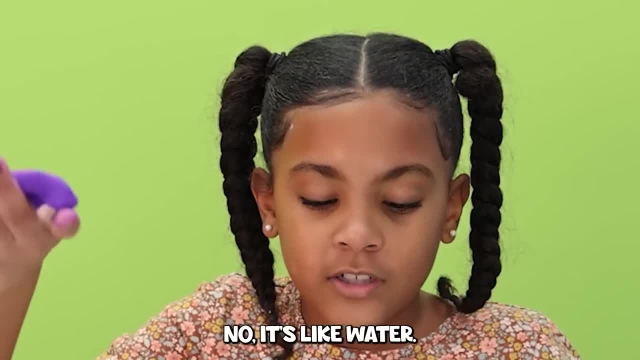 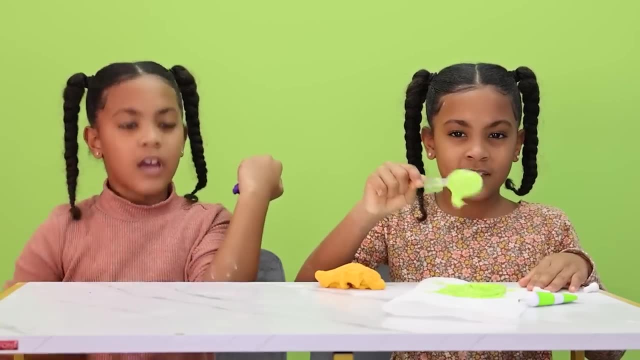 Oh my gosh, it's like thick water. No, it's like water, It's just. it's like. this is exactly the texture of icing, but I don't like icing. See, I hate icing. So this is not what I was expecting.